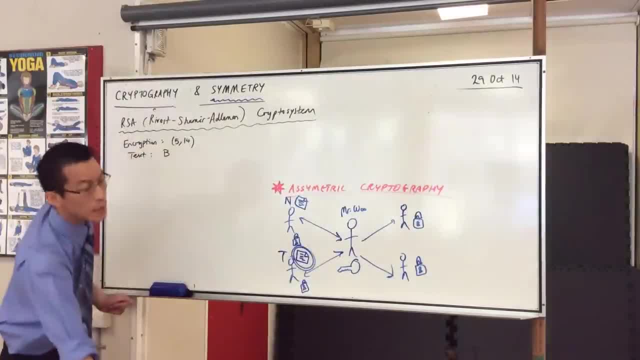 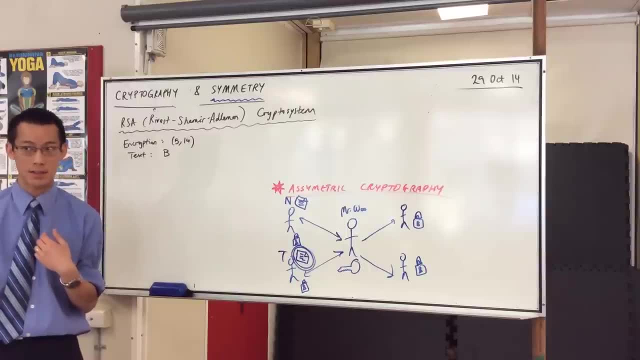 It's cool. Oh, my blood Alright. so how do we do this? Let me show you the maths of it. deceptively simple, But you do need to remember a little bit about what we did with modular rhythm, But it under the Caesar cipher. I promise it would be a heart, Okay. so here's what we're gonna do. 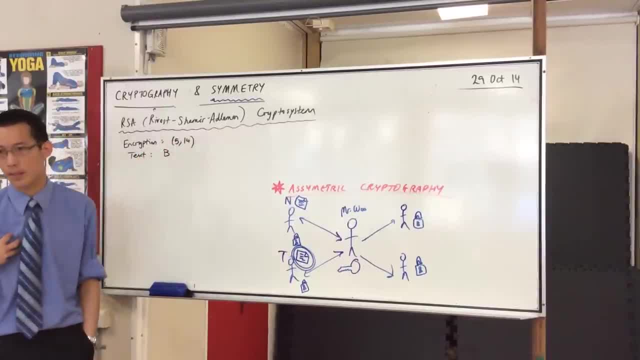 First step. this is: this is text, but we need to deal with numbers, right, So I'll convert this to a number. Okay, so, numerically, like we can decide on whatever, but I suppose we would call it to, wouldn't we? Okay, so to. that's the actual, that's the text, the number we're going to send. Okay. 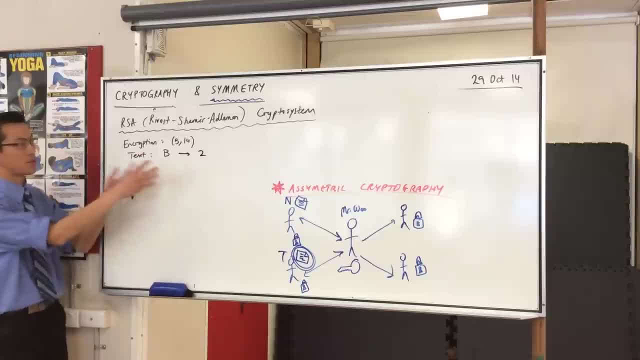 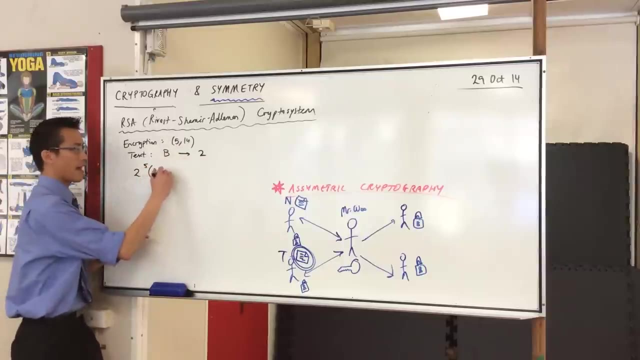 now I want to, I Want to use the cipher on this thing. Okay, so I'm gonna do is I'm gonna take this number two. I'm going to raise it to the first power, the power of the first number. I should have said right, so to the power of 5, and then I'm going to say mod. 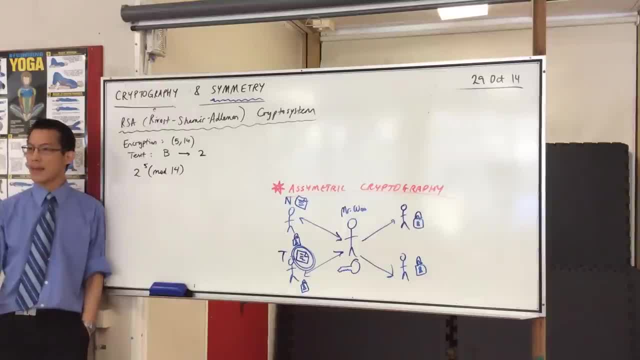 The second number. Okay, This is what I'm going to calculate. This is how I'm using the numbers. So, for instance, if you set the letter C, it should be 3, then what you would calculate is 3 to the power of 5 mod 14. 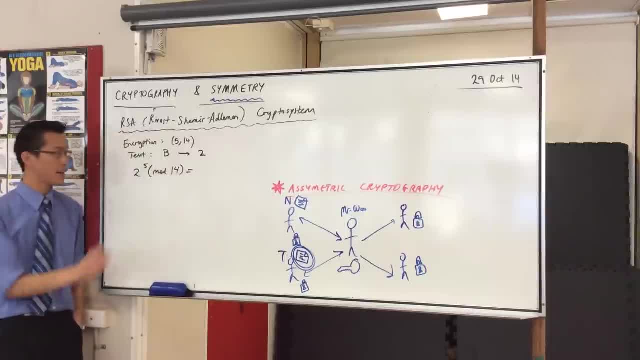 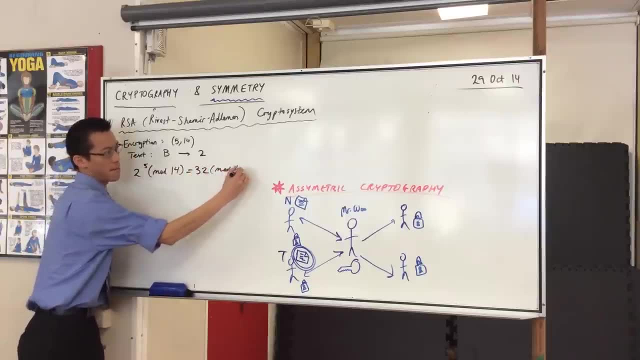 Okay, let's just quickly do this because the numbers are okay. This is how I chose them, right to the power of 5 To tell us that's 32. good, Right, mod 14. now do you remember what mod means? modular arithmetic right. 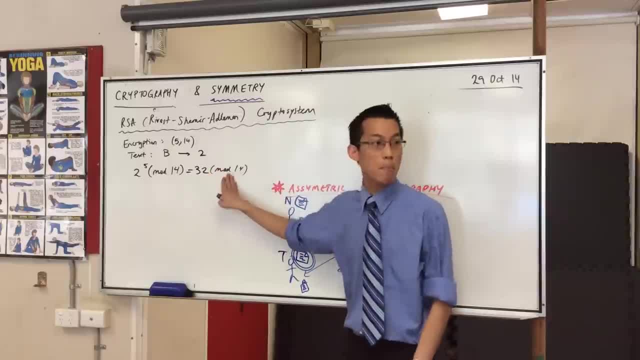 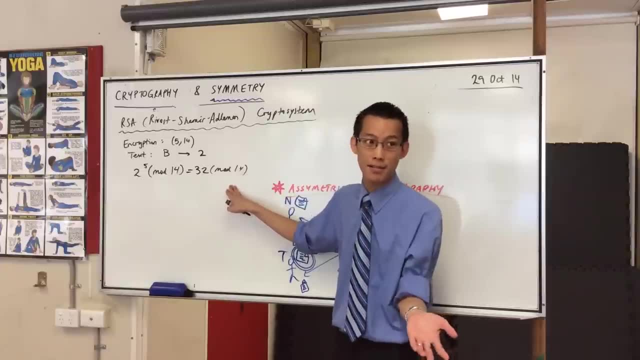 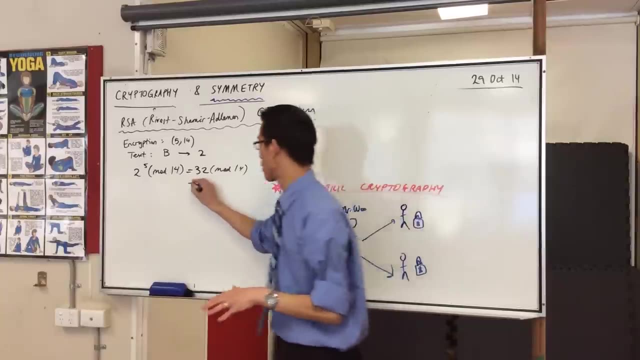 This number, 14, is called the modulus. what I want is the remainder that I get that's left after I divide 32 by 14. Okay, so of course, the biggest number, the biggest multiple of 14 you can fit into this is 28, And so what's left over is 4. does that make sense? Yeah, Okay, so that's a 4 mod. 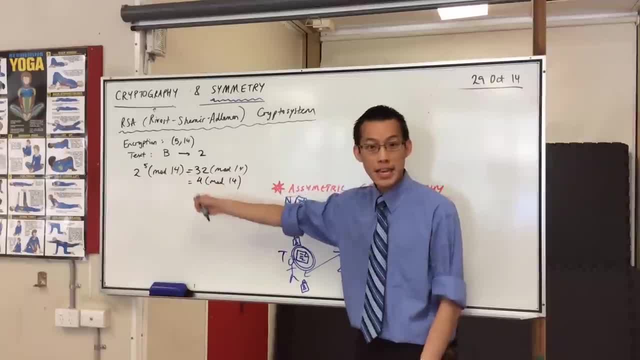 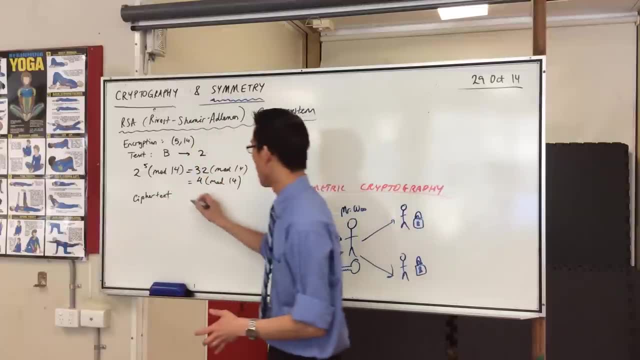 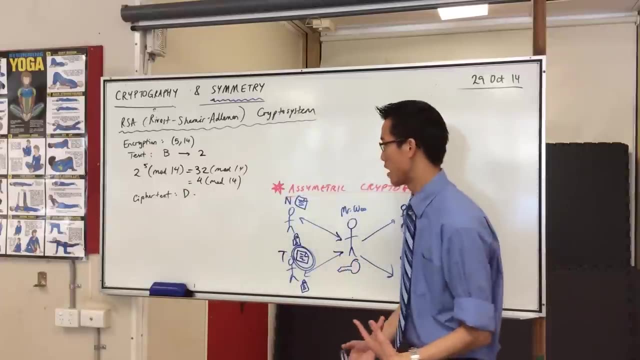 14. okay, so now for this is my cipher Text. okay, so the ciphertext, My encrypted message, okay, will be 4, which is D, I guess. So that's what you send to me, right, and now it's a secret. The original message is lost. 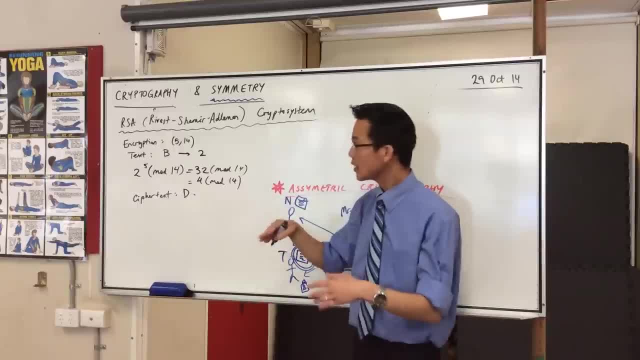 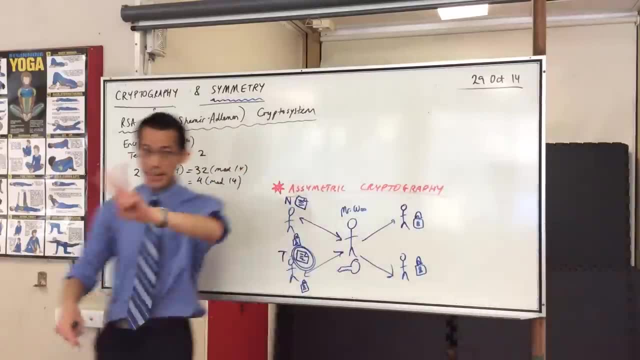 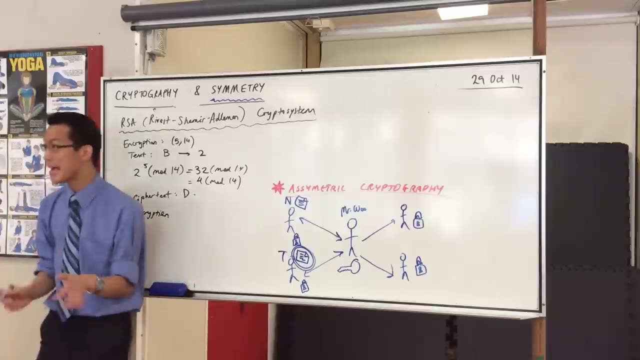 How do I decipher this? Okay, Well, You don't use this pair of numbers. Okay, I have the. I have the key, right? the key is related to this. the second number, the 14, is the same, but for Decryption the first number is different, right? So in some sense is this first number, It's the secret. 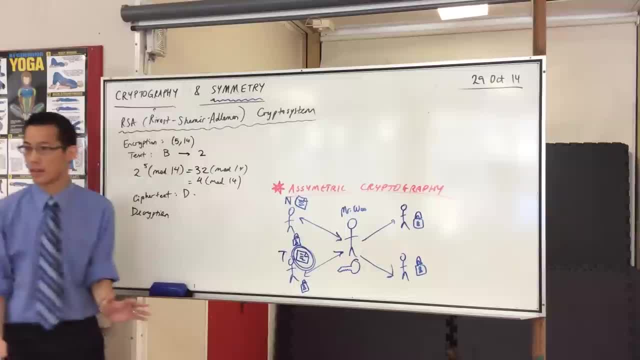 It's the, it's the key. If you find it out, you can decipher everything that comes to me. Okay, so in this case, The decryption key is 11, 14.. Like I said, this number here, the modulus is the same, But this number here, this one, is the key. 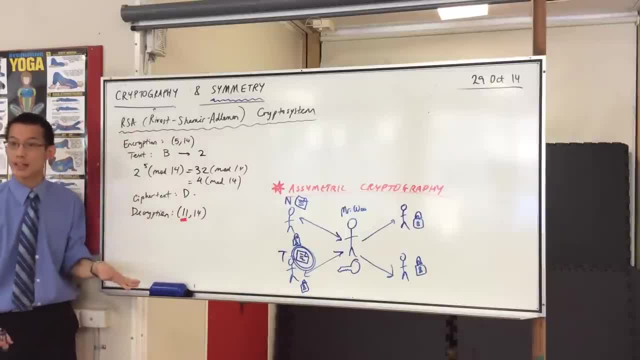 Now, what do I do with this? Well, I'm going to go through the same process, but I'm going to use this pair of numbers instead of This pair of numbers. Okay, I take your ciphertext right, Which was the letter D, and I'm gonna go through this whole process again. 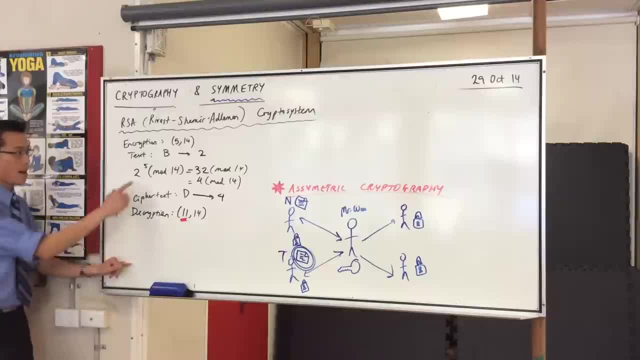 I have to convert it to a number which is 4.. Okay, then I raise it to this power and I say mod 14. okay, now to the power of 5. you could do that in your head, but for the power of 11, maybe not. 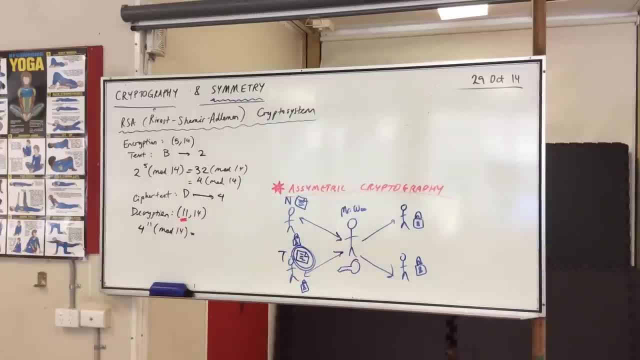 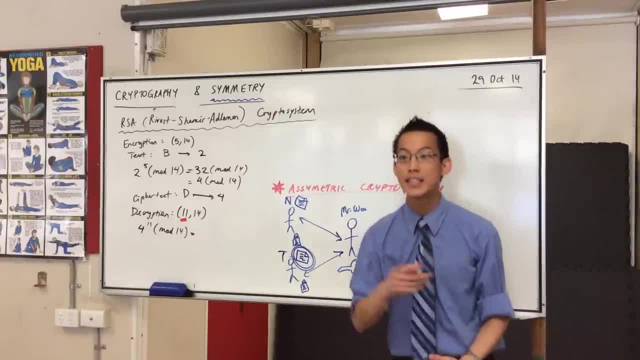 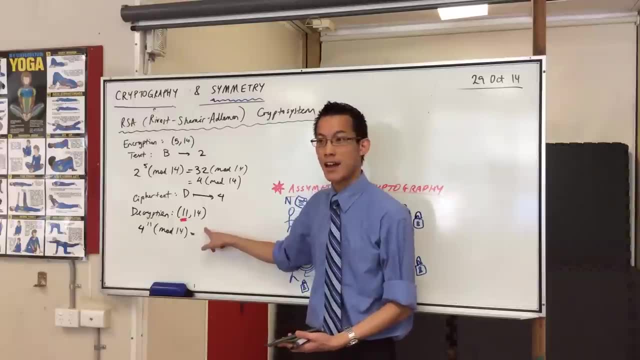 You get 11. I'll get to that, But the point is, I know what it is and you don't. That's part of the point that you can't just. you can't just see. Oh yeah, 5 means 11, right, The point is that no one can work it out. 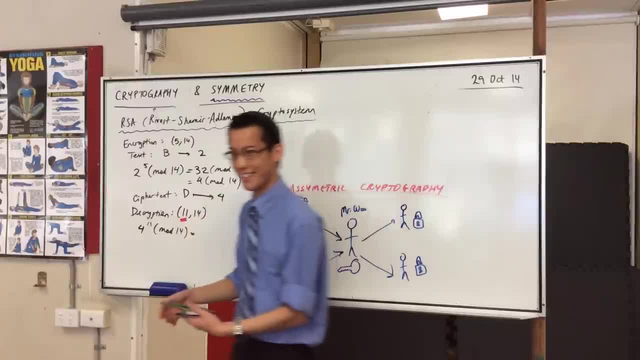 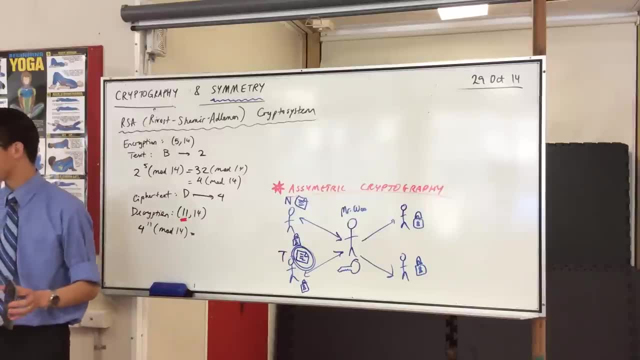 In fact it's all show. I'll tell you how hard is to work out in here. So I am this. yeah, No, and you'll think why. if it was always going to be 11, it'd be a pretty lousy description. All right, so you've got your calculator there now. yeah. 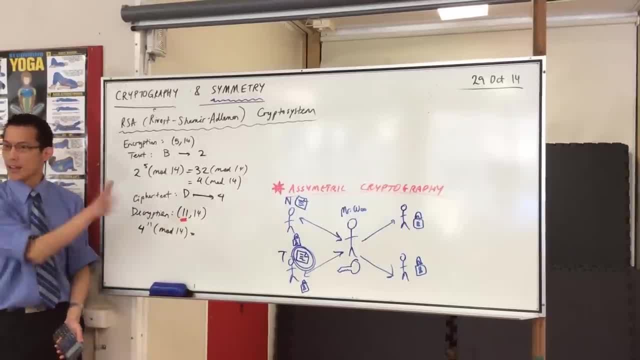 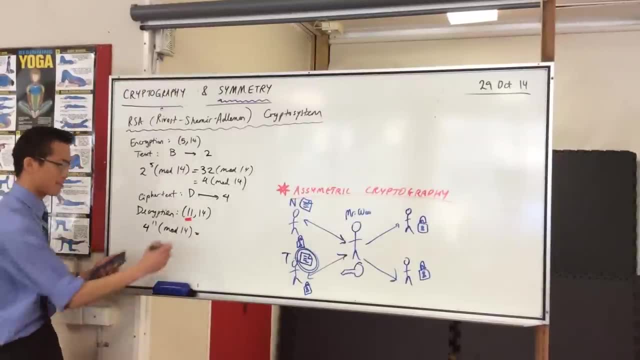 So the first thing you do, shh, the first thing you do- is 4 to the power of 11, okay, 4 to the power of 11.. Okay, now, then you get out this monstrous number, right, Okay, and this is mod 14.. 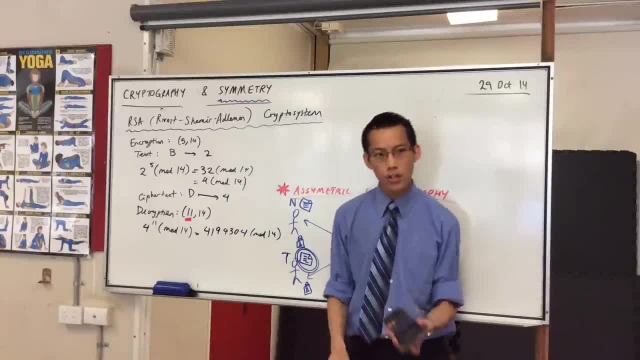 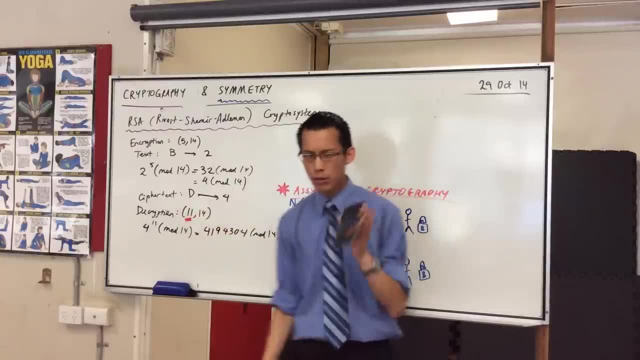 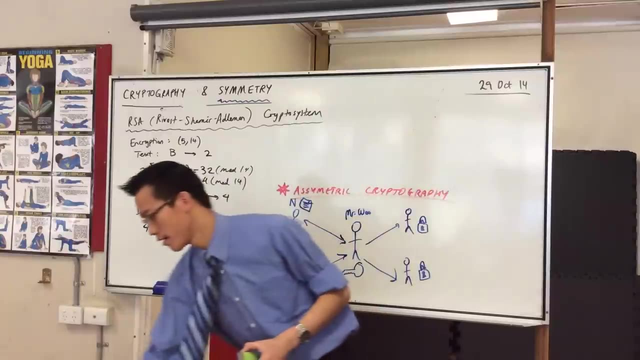 Okay, mod 14, right. So unfortunately, or maybe fortunately, our calculators don't have a mod button on there. Okay, so I will show you a sort of quick and dirty shortcut that will work out what this number is And actually part of your homework. I'm going to make a star here so that I don't forget it. 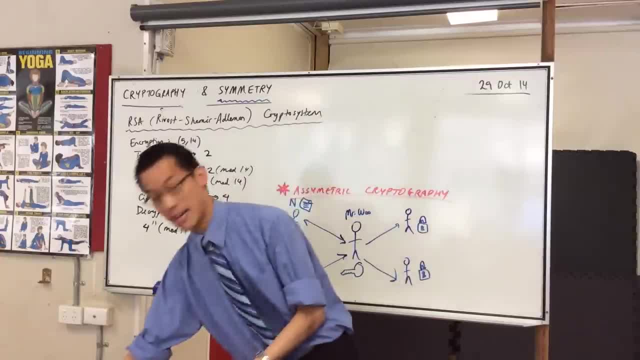 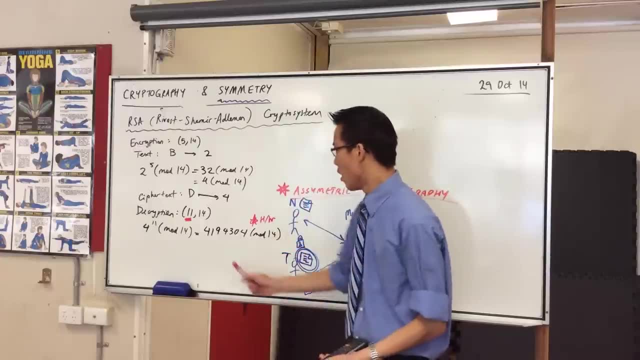 Part of your homework, in a post after this lesson, is to explain what I'm about to do, So you want to take note of what I do fairly carefully, okay, Why does what I do? what is? why is what I will do? why does it work? 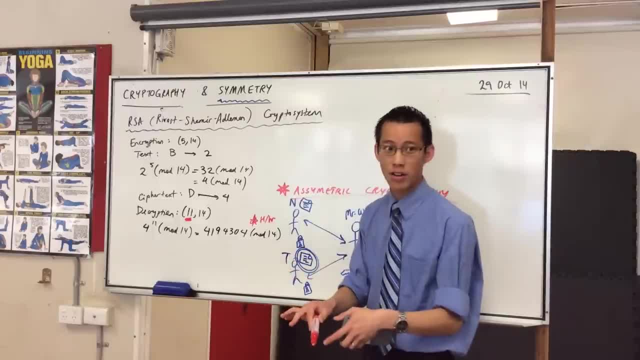 And it introduces: there's a problem with the number. It's easy to solve, but I want you to work out number one: why does it work? Number two: why does it introduce this problem? It's a strange kind of problem. 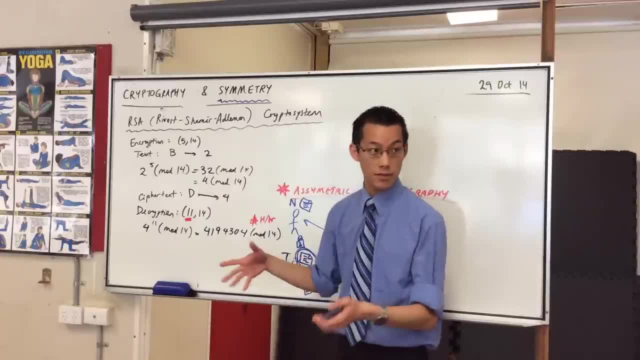 All right. so here's what we're going to do. Remember, this is about remainders, right and division and all that kind of thing. So the first thing I'll do is I'll take that number which is on my display and I'll divide by the modulus 14.. 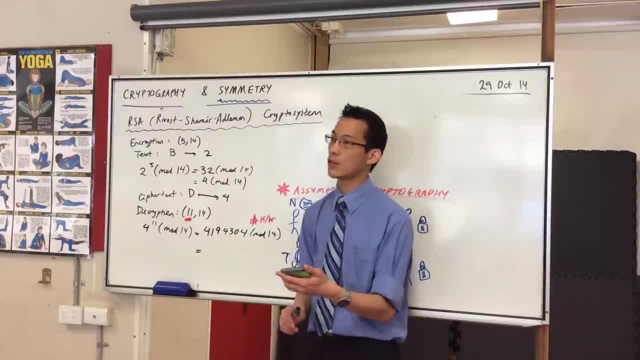 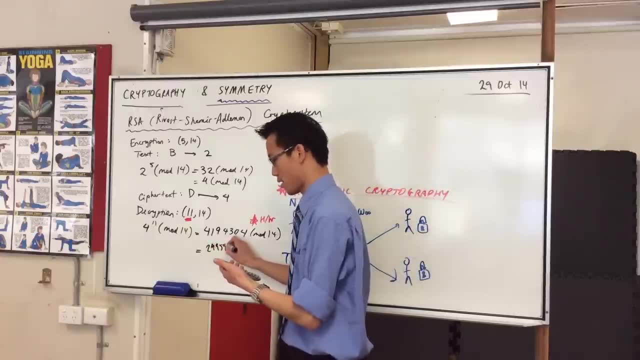 So you divide by 14. And it'll give you like a mine, gives you a fraction, but I want the decimal, okay. So this shows me 299593.1429, blah, blah, blah, blah. Okay, so I see that number, okay. 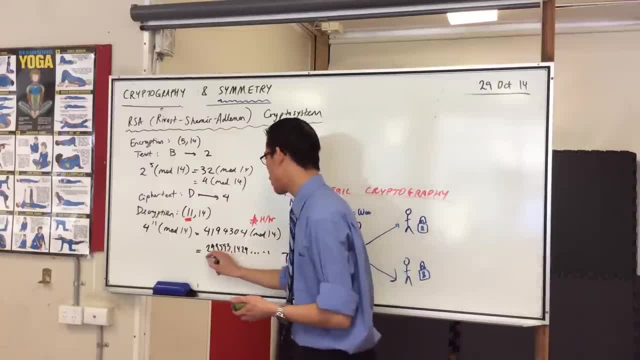 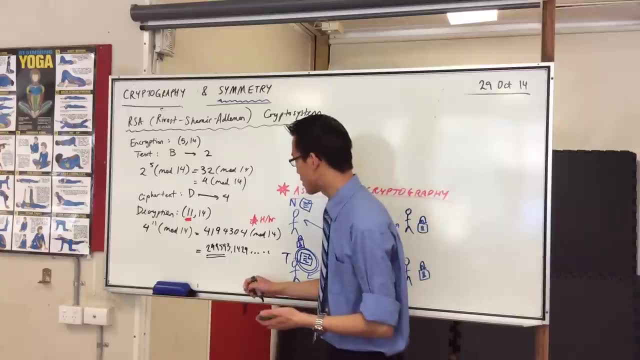 Now what I want to do is just mentally take note of the integer part of that number, which is 299593, okay, So what I'm going to do is I actually should have put that off on the side, but I'm running out of space, so anyway. 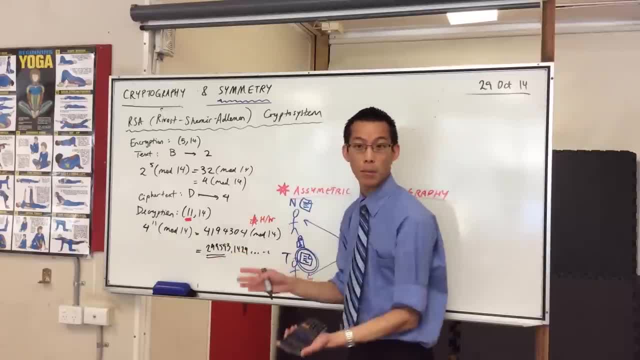 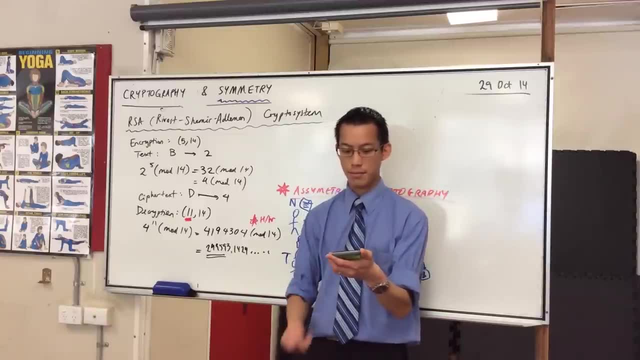 What I'm going to do is I'm going to subtract the integer part from the whole number. okay, So on my calculator, with this on the display, I say minus 299593, okay, And what's left is a decimal. In fact, it's this decimal. 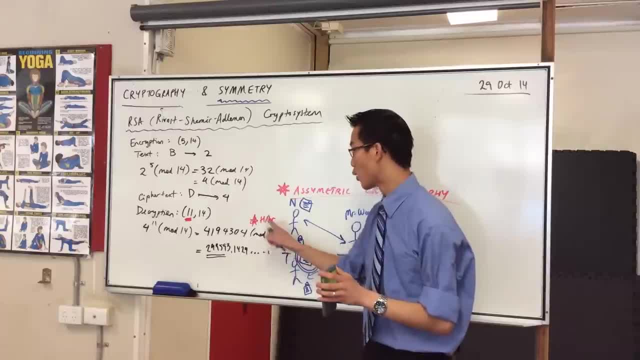 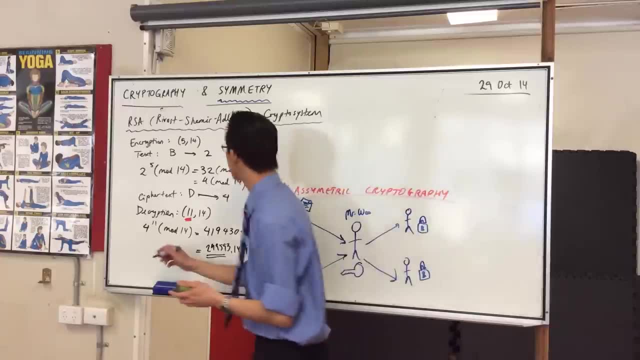 Okay, Now, once I've got that decimal there, I want to multiply back by this modulus 14,. okay, If I multiply by 14, what my calculator then says is: where am I going to put this? My calculator then says this: 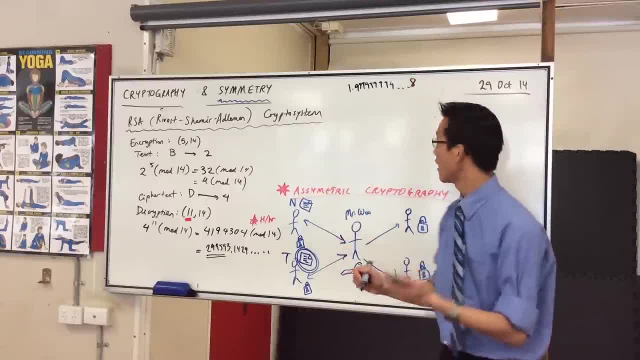 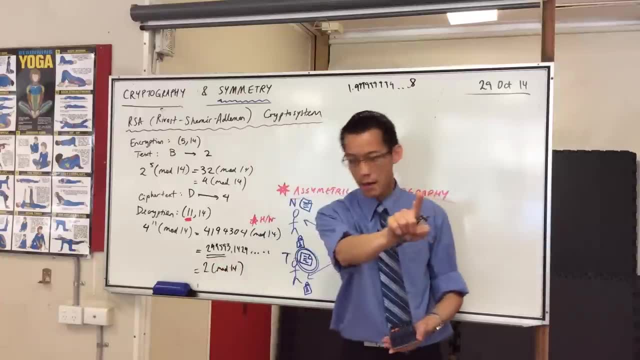 And there's an 8, or a couple of 8s on the end. okay, Now what number is this close to 2.? So this is 2 mod 14,. okay, Let me just remind you what's going to go in that homework person. 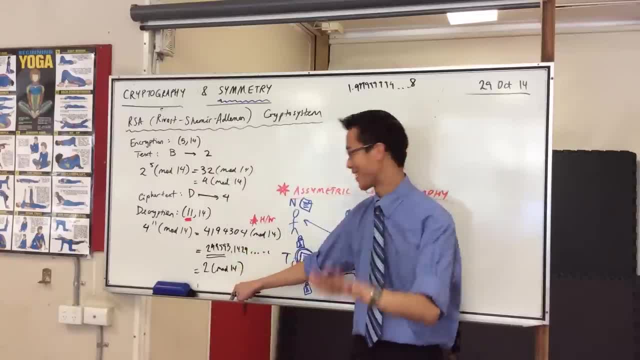 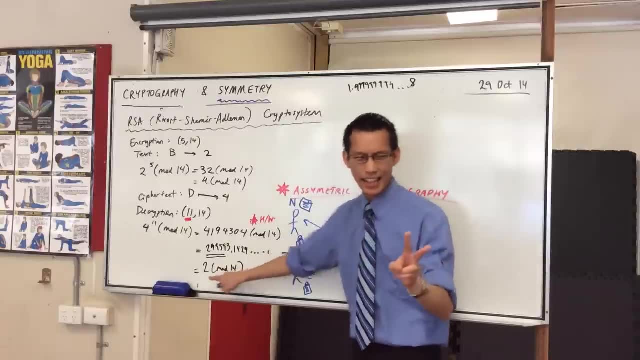 Number 1,. why does this work? That's not the hard part, okay. Why does this spit out the correct? this is called the residue, what's left over- okay. Why does that work? And secondly, why does it do this? 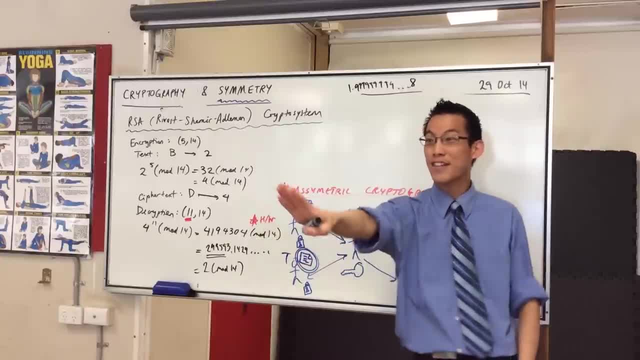 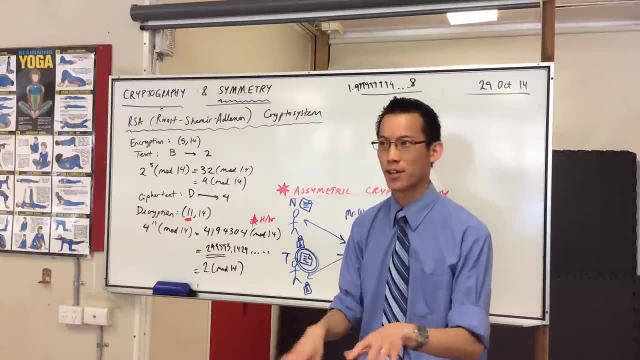 You think about it, You can work it out. okay, That's going to go into your homework. If you have an answer, No, there's an easy way to do it. I know there's an easy way. This is a particular way that it would be for all of us to follow.